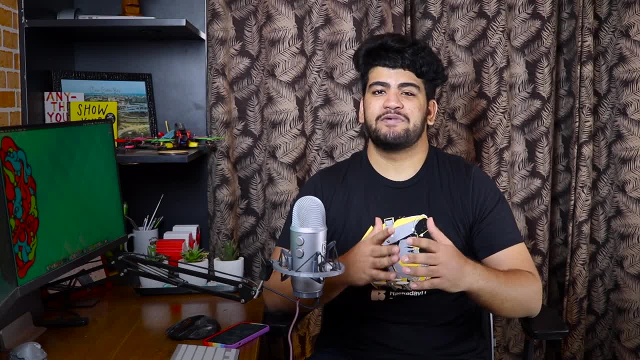 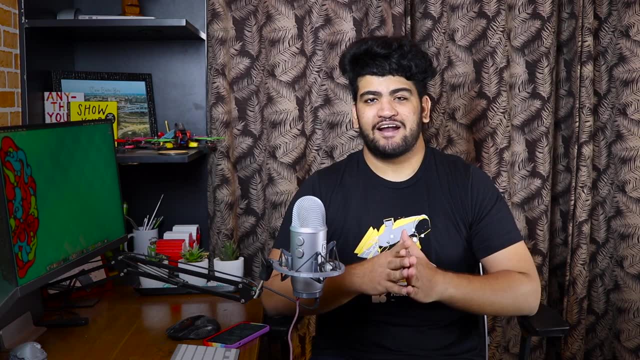 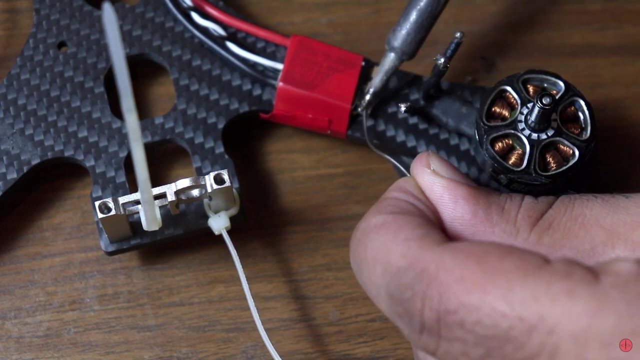 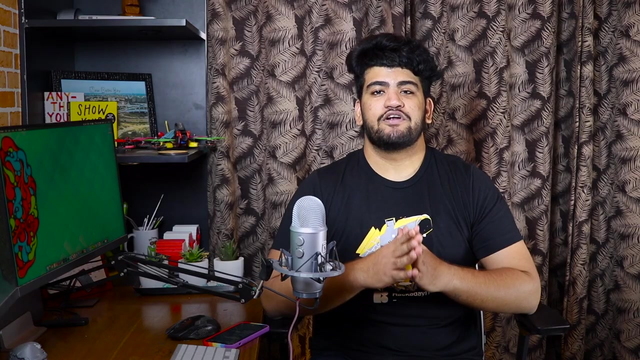 coming from technical background or not, should know soldering, because it's such an amazing and such a useful skill. And when I talk about soldering, I don't mean to do soldering by connecting two wires. That is a soldering. but apart from that, I am also talking about soldering components on the PCB, whether it's a through hole component, whether it's a small SMD component. so 0804,, 0602 and whatever, And I know it's not a very, very easy thing to learn and it takes some time. So how can one 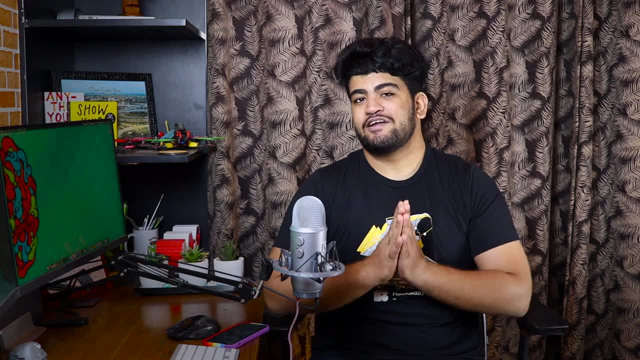 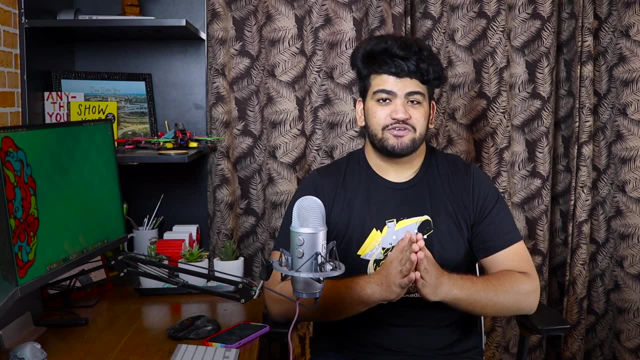 who have no idea about soldering can learn soldering. First of all, get yourself a good soldering iron. I made a video on a good soldering iron which you can get in budget. Check out the link in the description. So, once you have the soldering iron, there are a lot of different. 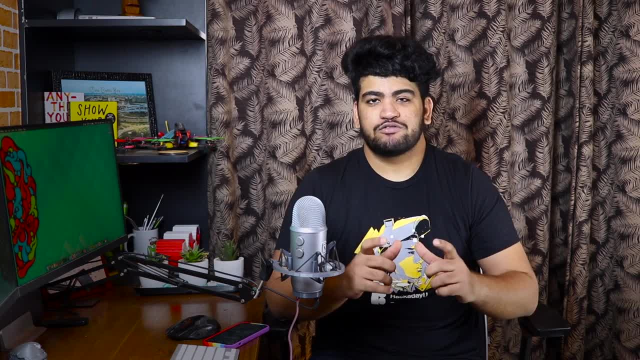 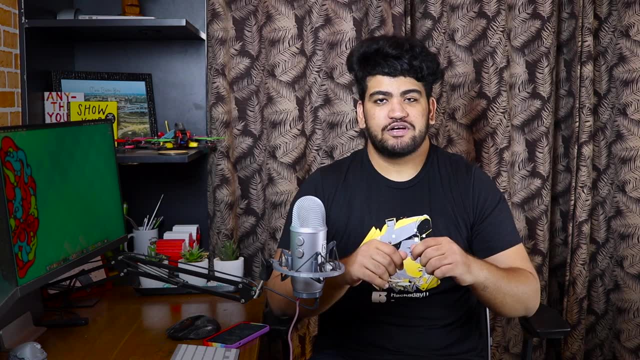 tutorials on internet which you can follow. You can buy some small soldering kits. These are the small PCBs which supplies you with the bare board and some components so you can solder on them and you can make something out of it. So you can find some of these kits on Tindy, which is my 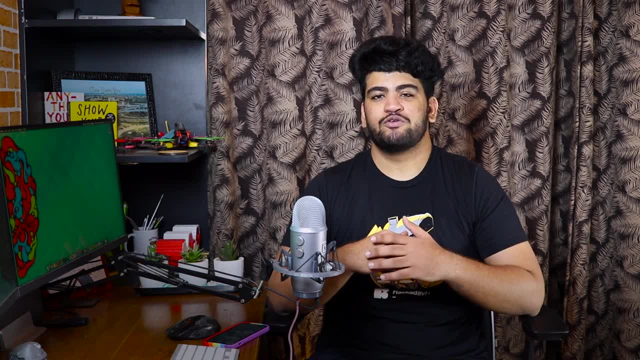 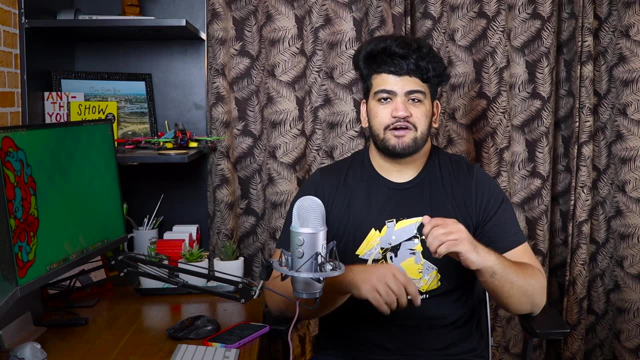 go-to site for getting these kinds of stuff. I'll leave the link in the description so you can buy it. You can also just buy the zero size PCB which has all these small holes, and you can start soldering resistors, capacitors and make something out of it. So that is one way to learn. 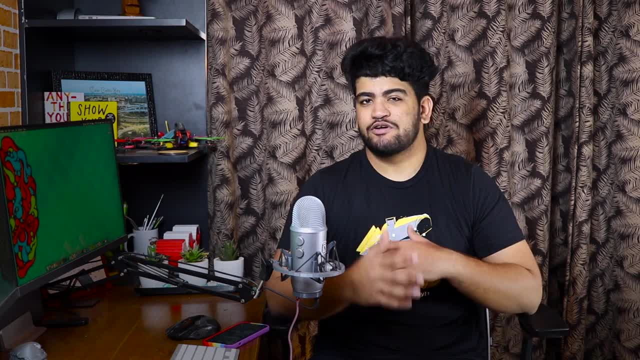 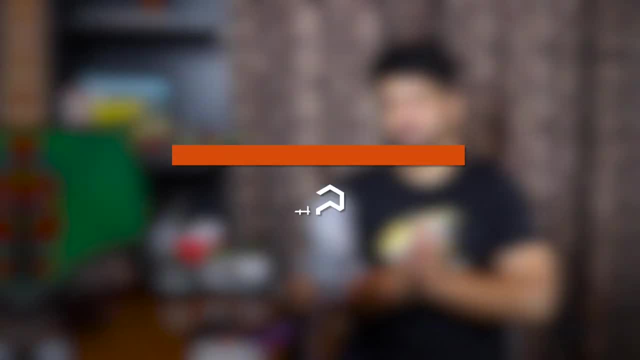 soldering. And as you do more and more on daily basis, your skills absolutely grows with you. So, yeah, that is the first skill on my list, So do learn soldering. Now on to the next one, that is breadboarding. Just like soldering, breadboarding is another skill which I think everyone from. 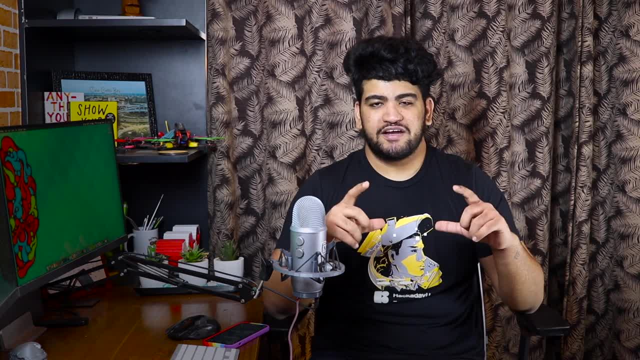 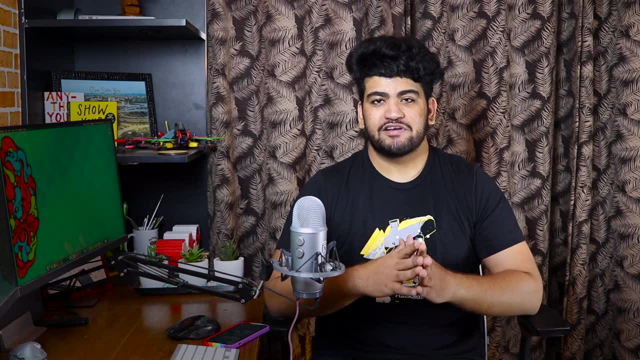 nice and electrical background should know. So what is breadboarding? Basically, it's a small rapid prototyping platform where you can design a circuit very quickly, prototype a circuit and you can just verify your proof of concept that the circuit is working or not. And it's a temporary. 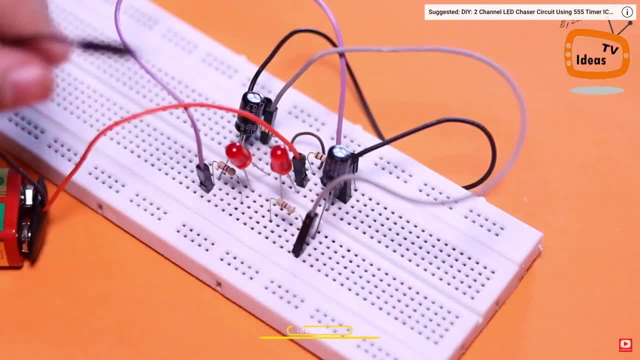 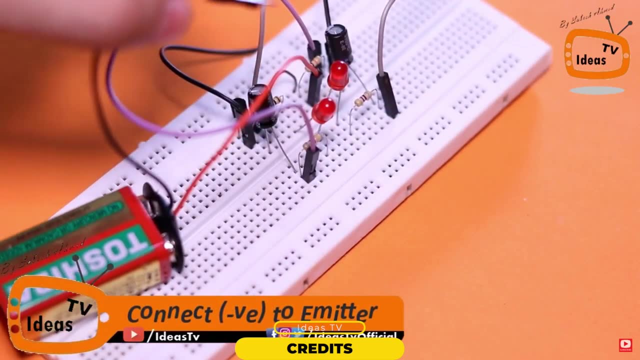 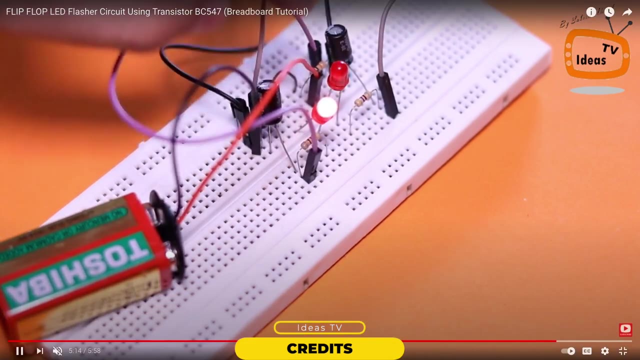 solution. so it gives you temporary connections and you can change it very easily And, unlike PCB where you solder everything once it stays on breadboard, You can change the components. you can change its circuit anytime. So this is the first step in any circuit design. Breadboarding is the 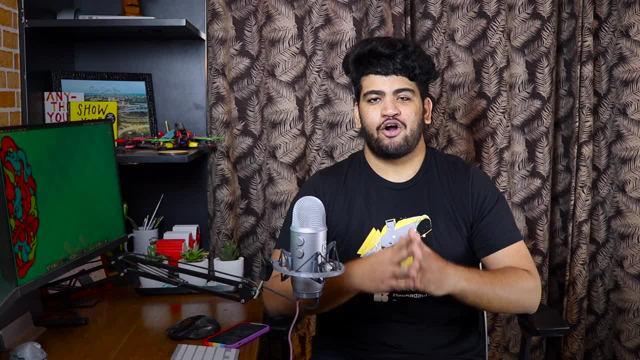 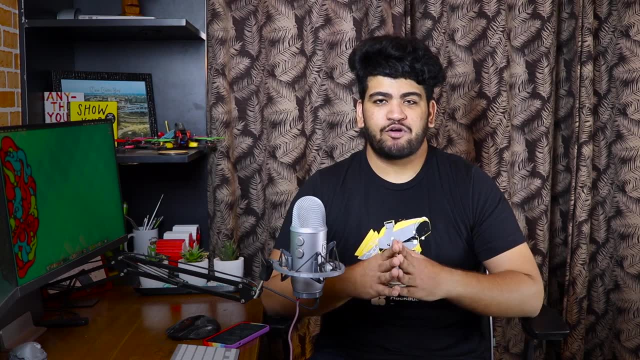 first stage of any circuit design, in which we prototype the circuit on the breadboard to see if it's actually working or not. And breadboards are not very costly. you can buy a good breadboard in 70-80 rupees. You can get it from Amazon. I'll leave some link in the description, as usual, And 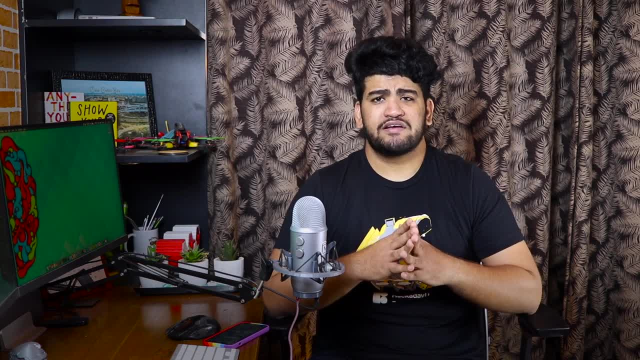 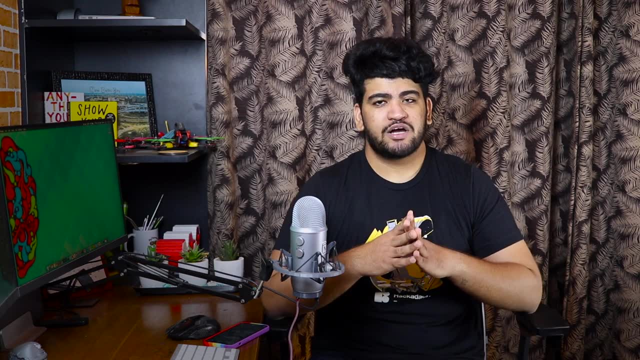 yeah, learn about breadboarding. There are tons of different tutorials out there on Instructables, even on YouTube, that how a breadboard is connected, how you can use, start using a breadboard. so, yeah, that is another skill, in my opinion, which you should know if you're coming from. 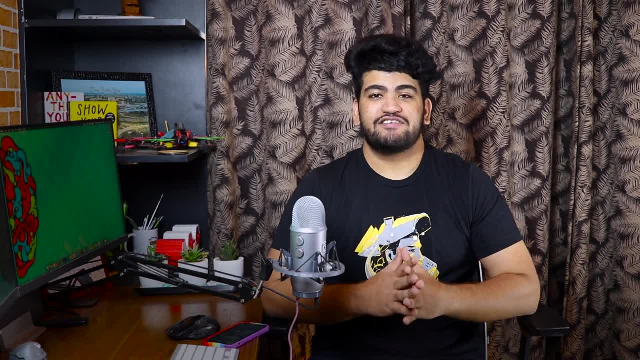 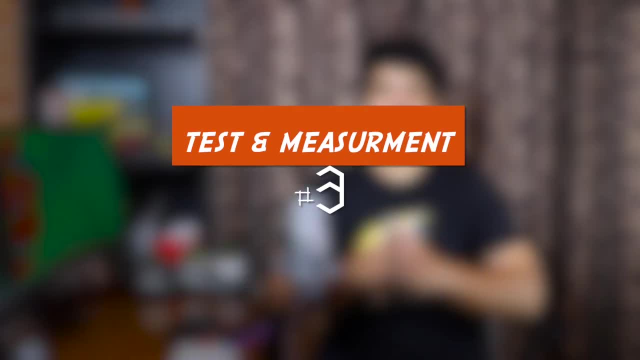 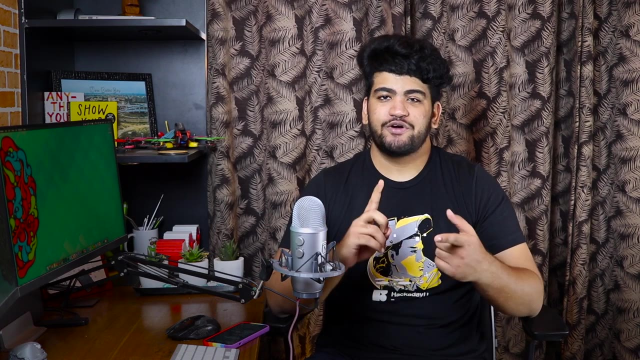 electronics or electrical background. moving on to the third skill, which in my opinion is really important if you are from ec or w background, is using test and measurement equipments, and what i mean by using tnm equipments is using multimeter logic analyzers, cro, dso and all kind of stuff. 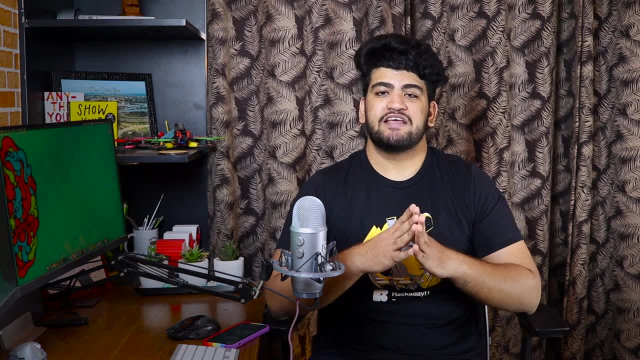 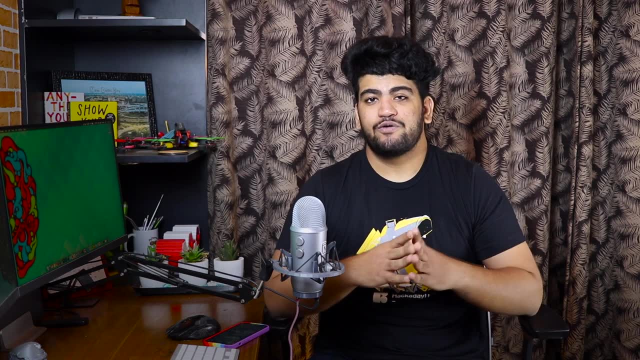 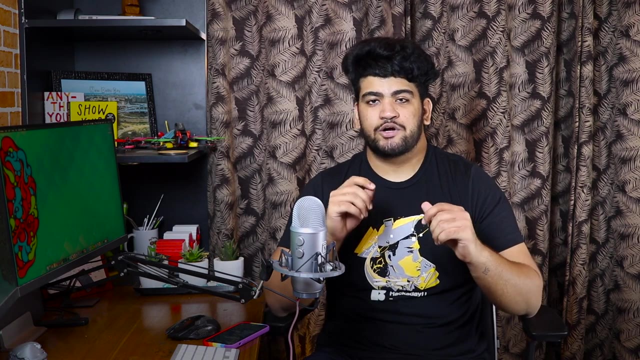 so we need to use all these equipments. there are tons of different possibilities where you can use a multimeter logic analyzer or cro. so, for example, a continual test will tell you using a multimeter that two points are connected together or not. similarly, if your circuit is not working and you 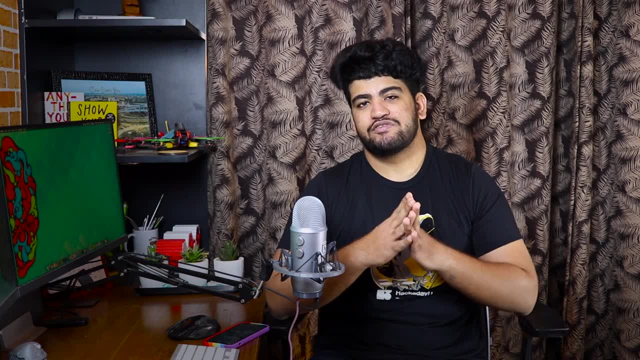 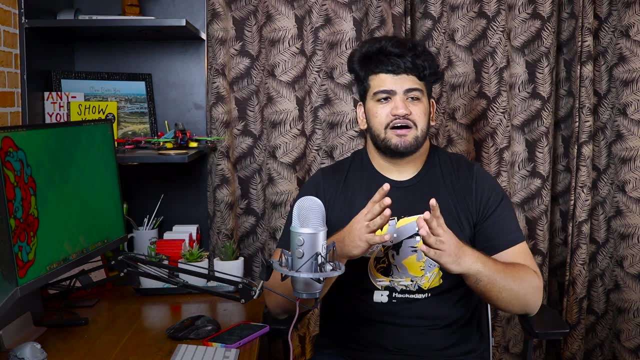 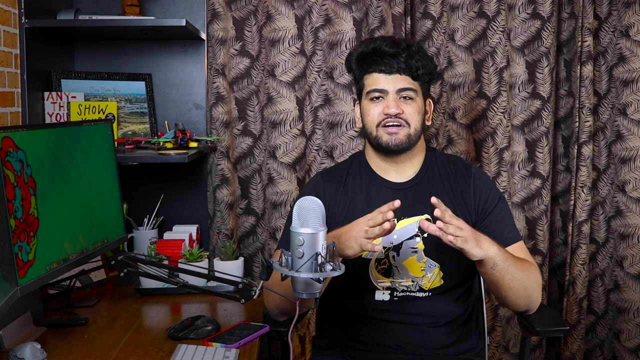 need to just debug it. you can use a cro to see if the waveform is coming or not, if it's a right waveform, the frequency, amplitude and similar kind of things, similarly using a signal generator, a probe in cro, all kind of things that comes under, using tnm equipments and uh. you can follow youtube. 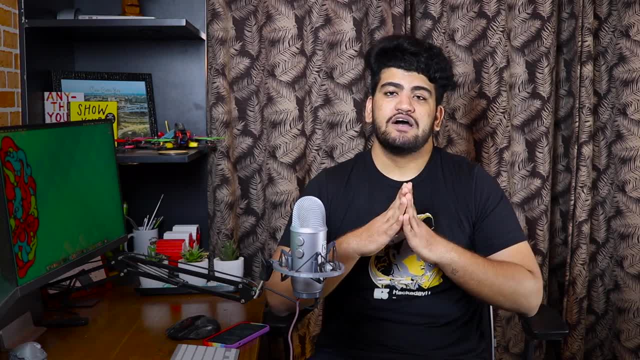 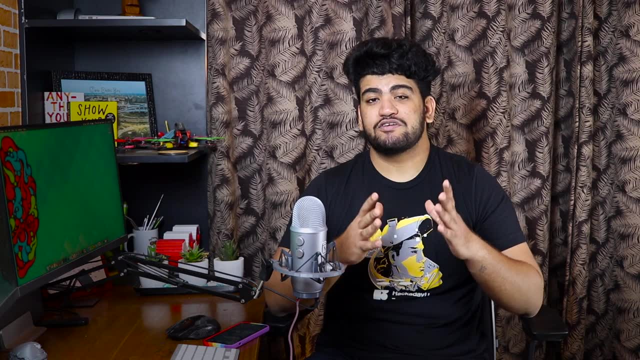 tutorials. there are tons of different videos out there which will teach you how to use a cro, how to use a multimeter, and everyone should have a multimeter. but cro is not that important these days because cro has uh can be replaced by something called logic analyzers. so 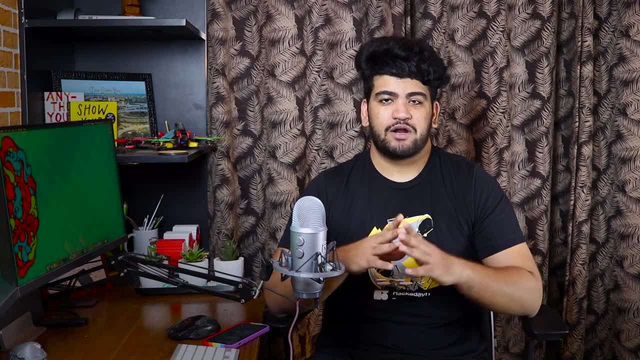 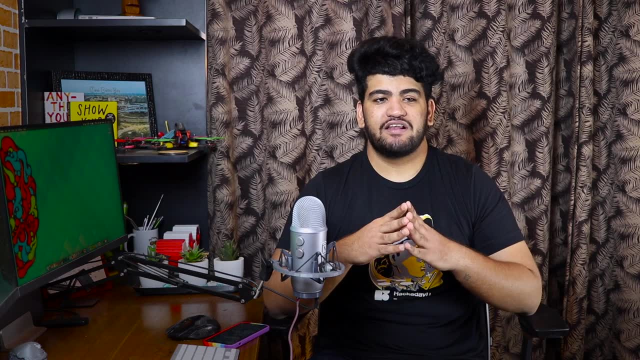 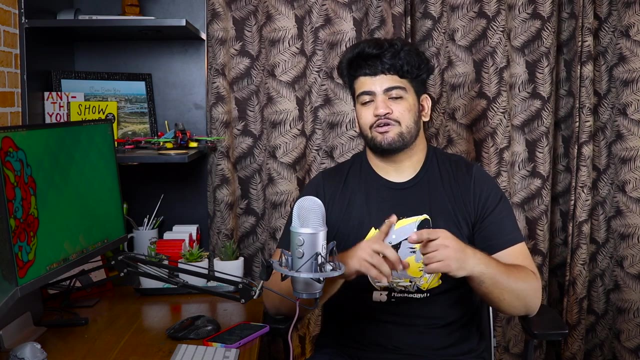 which you can purchase for quite cheap compared to the traditional cro. i know people who are into traditional electronics. they will uh prefer cro any day. but if you don't have a budget because cro are really expensive, uh, then you can either buy a second hand or go for something called. 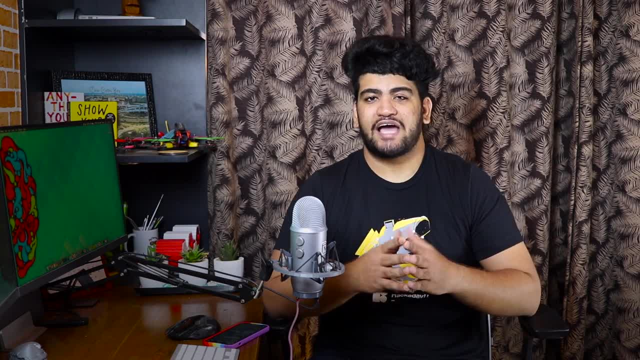 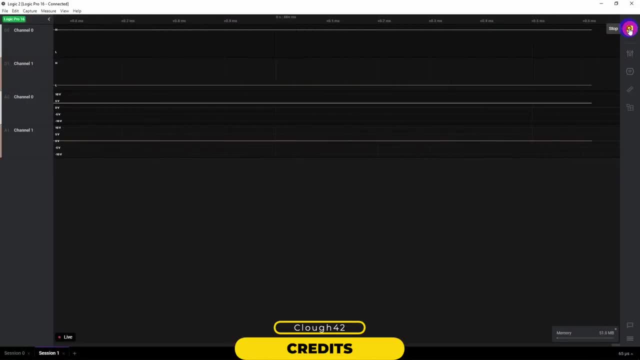 logic analyzer and the logic analyzer which i recommend is sally logic analyzer. so what it does? it connects to your computer via usb and it has some probes which you can attach to your electronic circuit and you can debug it on your computer. you can see if the wave is coming, the frequency. 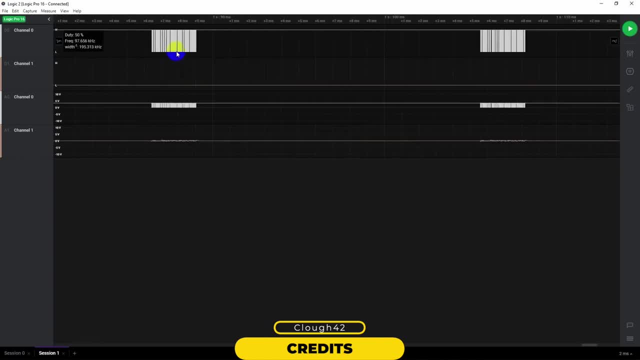 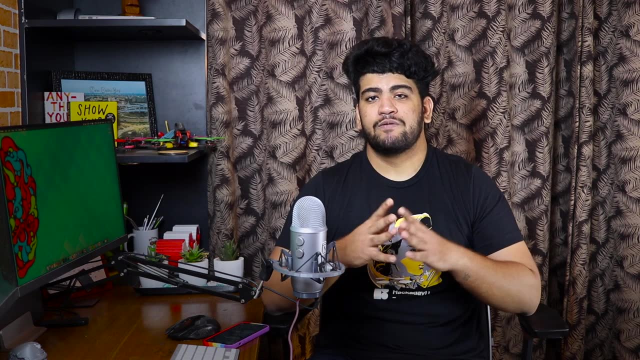 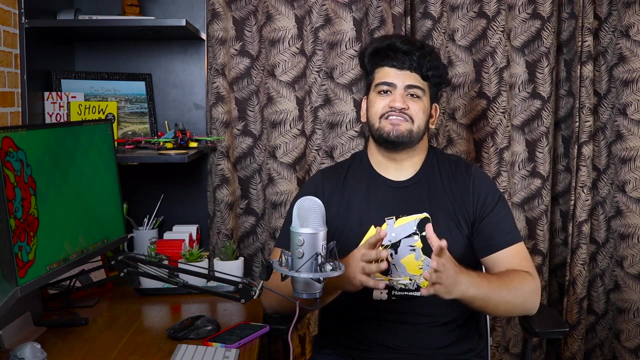 the amplitude and things like that. so, uh, that is a really important skill to have. it teach you circuit debugging, it teach you circuit reverse engineering and troubleshooting and all kind of things. so, uh, if you go in an industry and work for a professional setup where they design circuits and debug it, uh, these equipments plays a really, really important role, and one 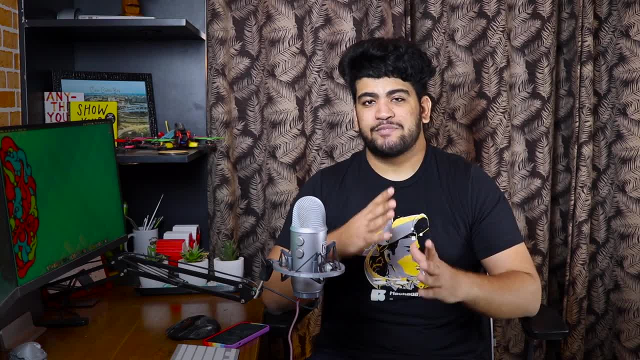 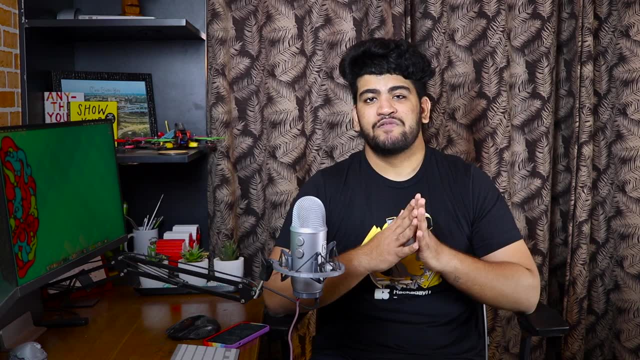 should know how to use them, how to use them correctly and what are the shortcomings of their equipment. so make sure to learn it before entering the professional life. if you are interested to make your career in electronics or electrical, that is something you need to learn. moving to the next skill, the number one skill is the circuit debugging. 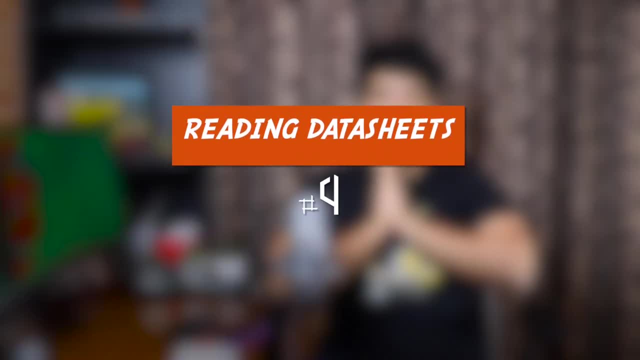 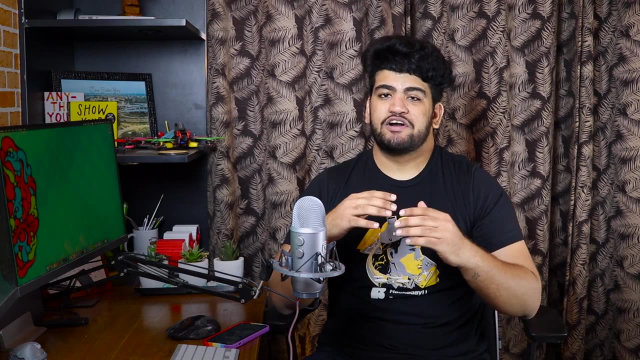 number fourth on my list is reading data sheets, and that is, hands down, the most important skill which i have personally acquired over the period of time. so, basically, what happens is when you are designing a new circuit or when you are working on a new project, you come across different components. 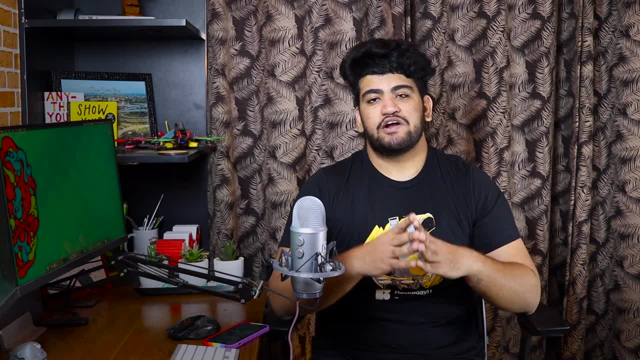 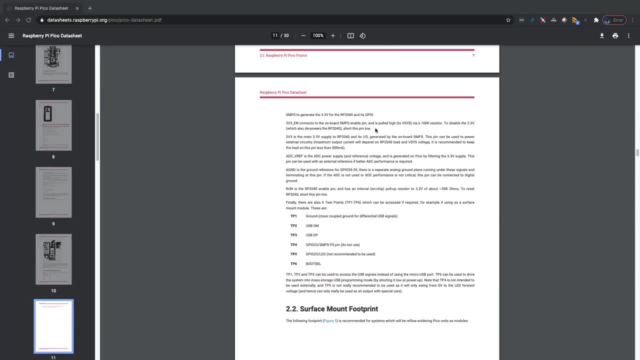 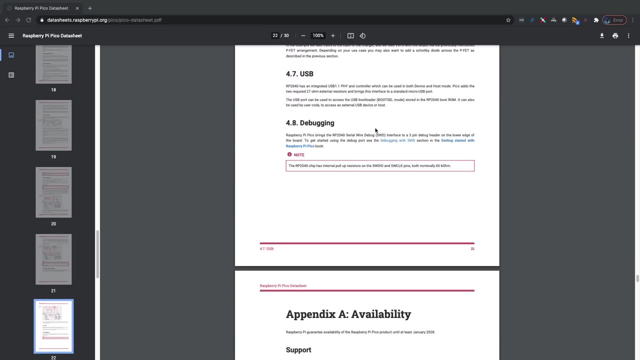 which are new for you, and the only way, the best way to know any component from heart's out to read, is data sheets. so every component, whether it is a passive component, whether it is an active component, whether it is a microcontroller or you want to know about its architecture, data sheet is the only. 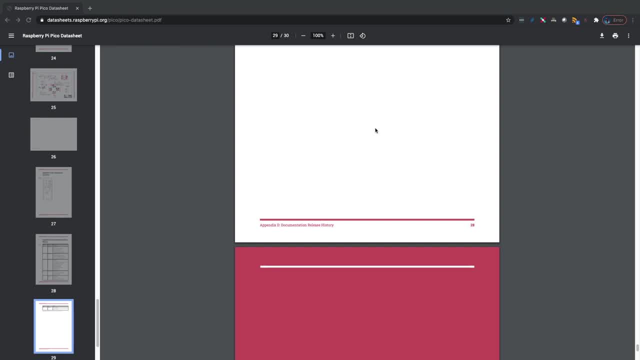 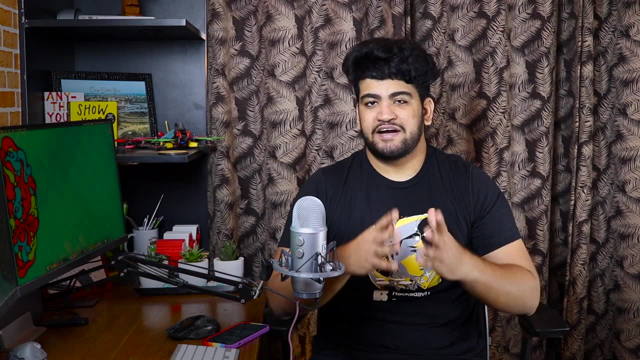 go-to source which manufacturer provides. uh, even, if you want the size of the component for pcb design, then the data sheet is the only way to learn it. so, uh, data sheets. obviously, manufacturer provides you with the component. you can download it from the internet, from their sites, and 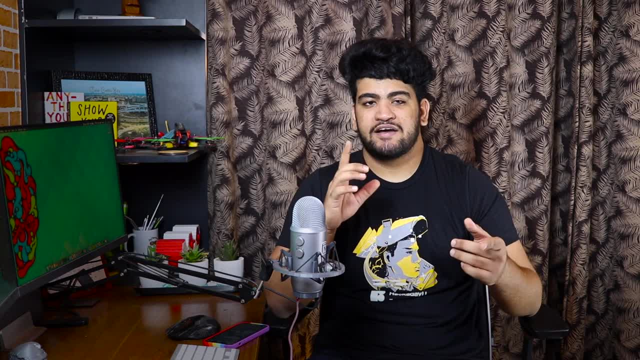 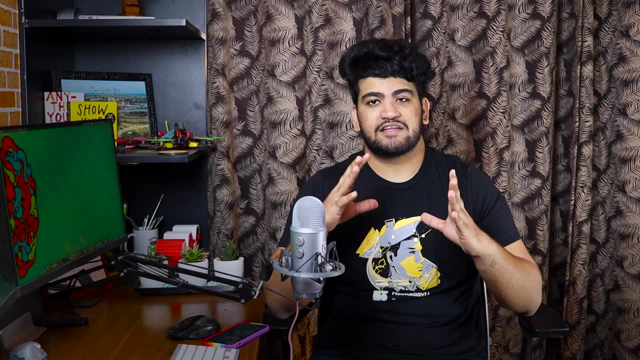 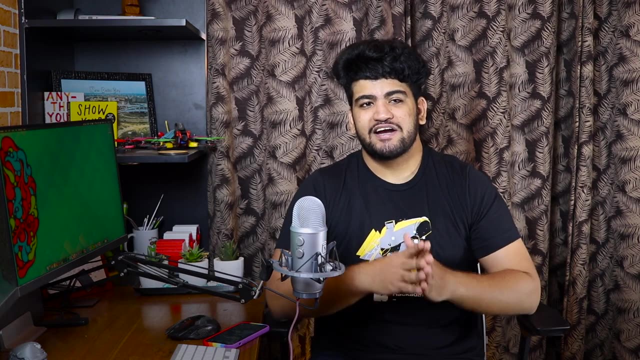 data shift tells you everything there is to know about the component: the electrical characteristics, the frequency characteristics, the uh environmental characteristics, the temperature of the environment can withstand, how much frequency it can work, uh, whether you need some decoupling capacitors with it, whether you need some support circuitry with it. everything will be there on data sheet, if you are. 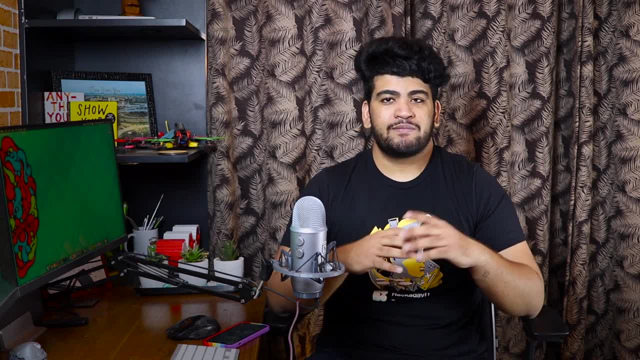 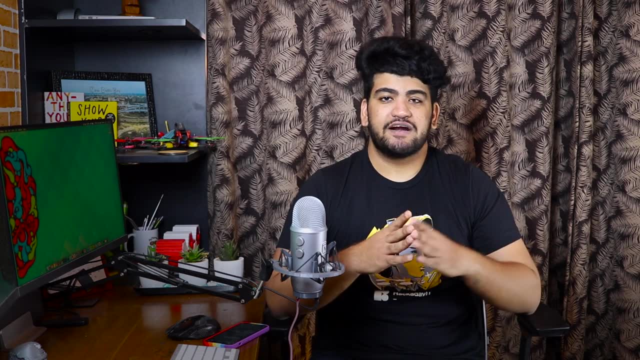 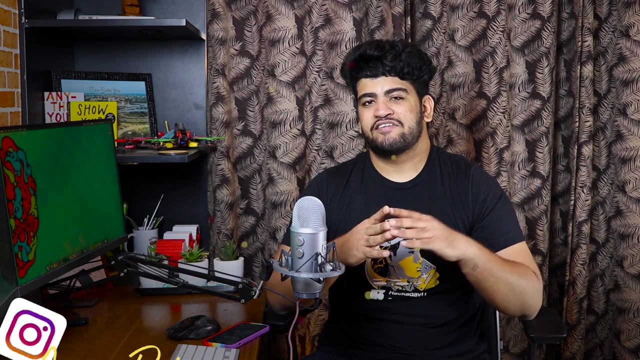 working in. uh, let's say it's a programming environment where you need to program micro controllers. then the reading, the architecture is: uh, cpu registers, uh adc. how much bit is it? watchdog timer, how it works. which flag to set will start its counter? which flag to set timer? 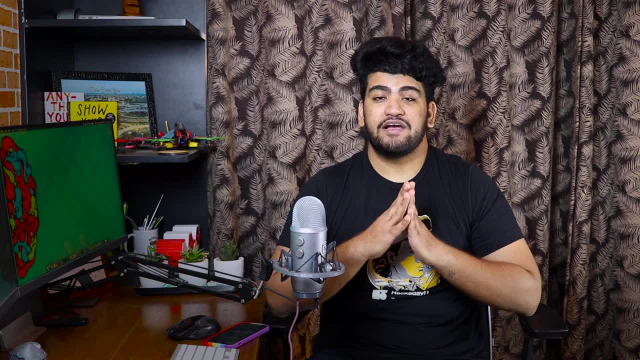 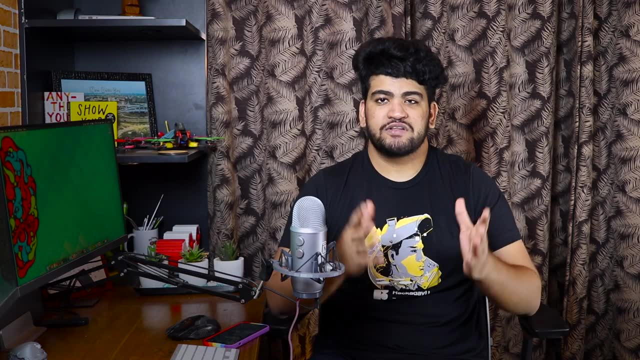 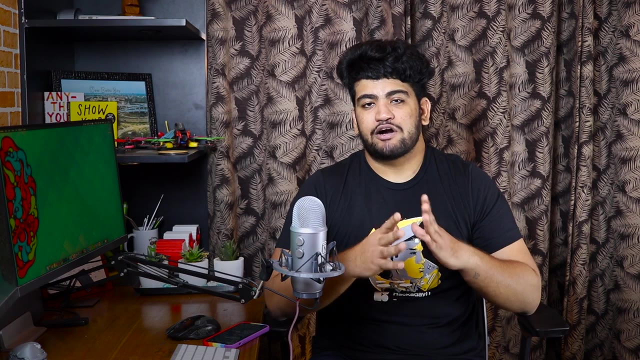 everything will be on the data sheet. so make sure you read a lot of data sheets, and there is no way to learn how to read data. you just have to pick the data sheet and use it as an encyclopedia. go to the page number which you are interested in about the part to know, and then read a lot of data. 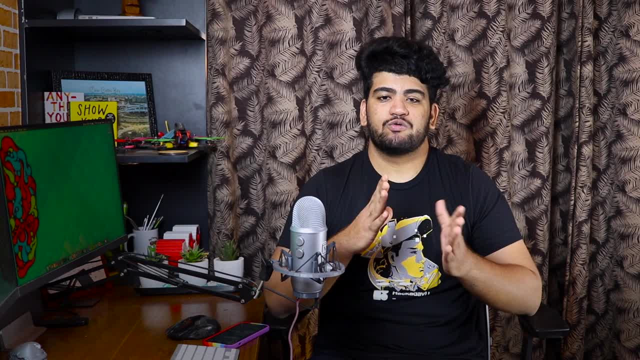 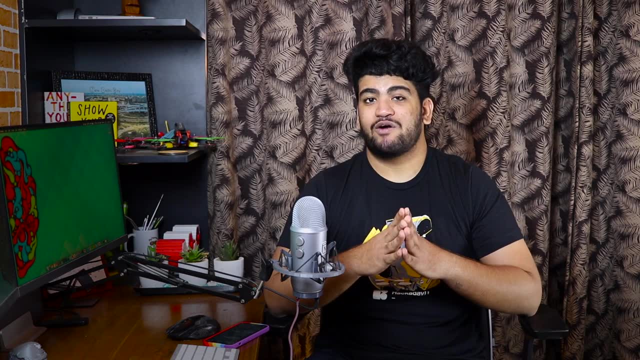 sheets, then only you will, over the bit of time, you will understand how to actually read a data sheet. so that's a very, very important skill in my opinion. if you want to make a career in electronics or electrical background, make sure you know how to read a data sheet of any component. all right, 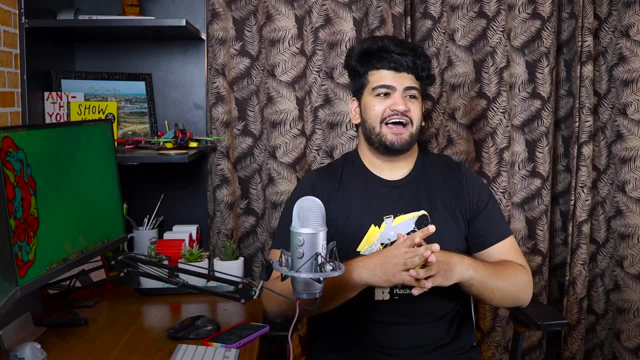 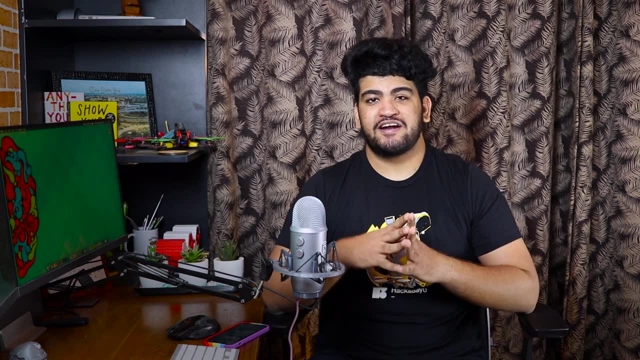 number five and the last one on my list which can be a bit controversial and polarizing is, uh, programming. so i know you people must be wondering that if i want to make a career in electronics and electrical background, where i will be designing pcbs, where i will be 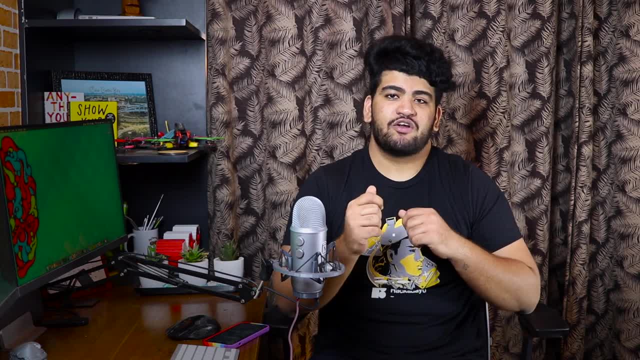 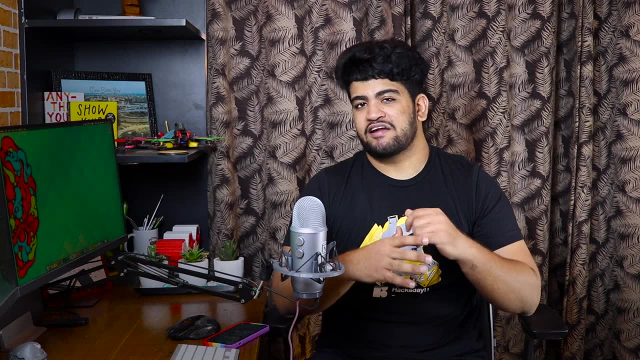 reading data sheets where i will be debugging some uh equipment using logic analyzers and whatnot. why the hell would i need programming for it? so? so hear me out. so programming is not just something that um and nerds of computer science background do. programming is like a tool in your 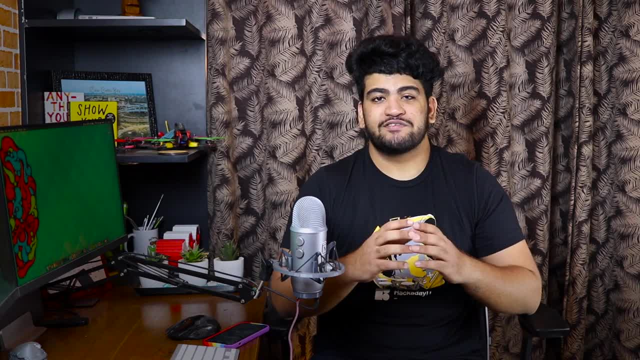 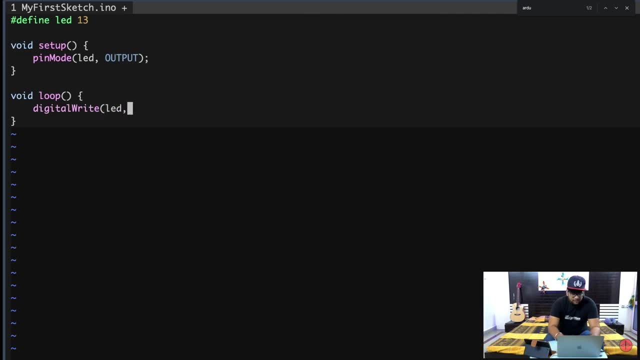 arsenal in your toolkit which will enable you to do so many different things, whether it's automation, whether it's testing, whether it's just simulating something. so programming seekhna is like giving you the opportunity to, which opens the door of lot of four different possibilities. 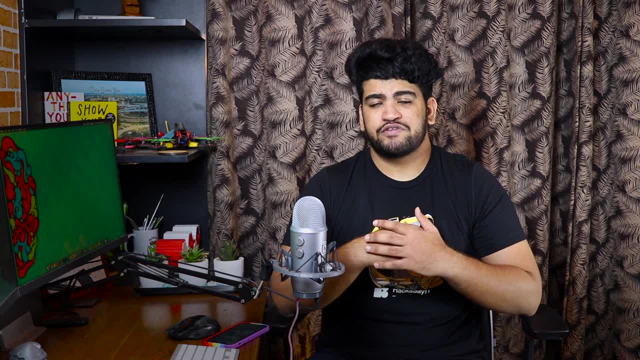 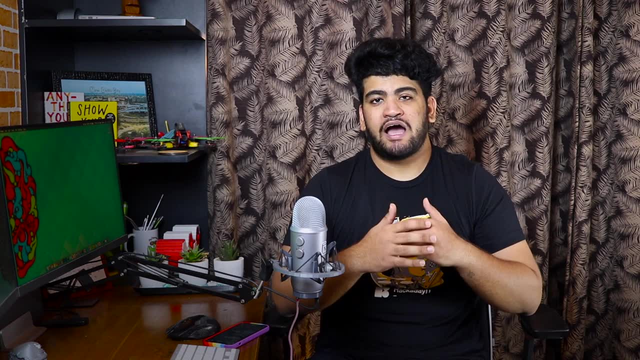 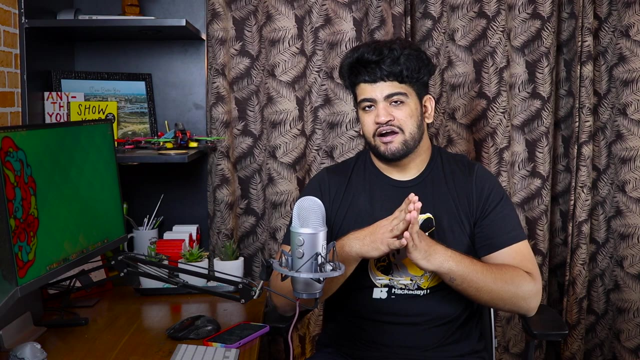 where you can. it's like a playground where you can do all kind of things. for example, if, if you, if you are doing a manual task again and again, you can automate it with programming and do it automatically, the computer will do it for you. for example, if you want to take a reading of, let's say, hundred different